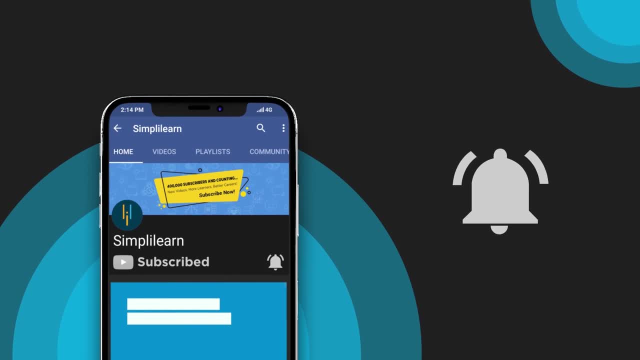 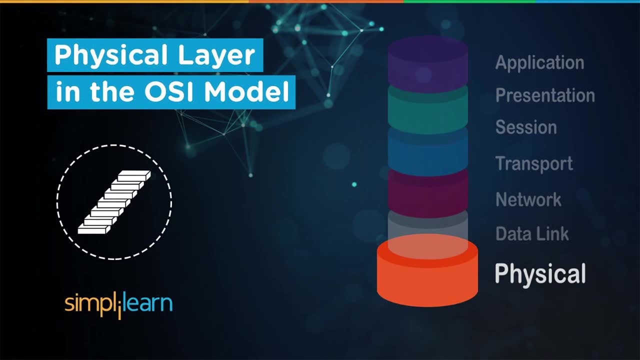 Have you ever wondered how data is transmitted through a network with the highest search traffic? Well, not to worry. Today's topic is everything you need to know about data transmission through physical layer in the OSR model. If you are watching this video, then you are a techie. 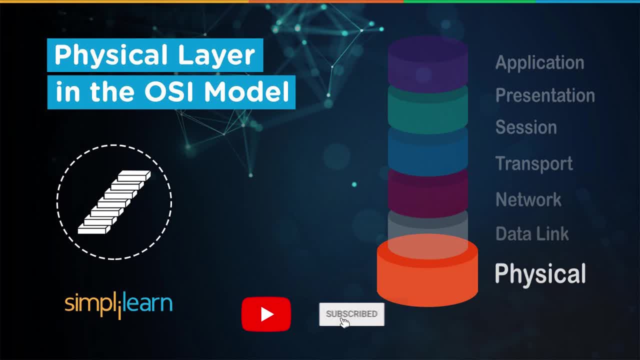 Love watching more tech content? Then subscribe to the Simply Learn channel and hit the bell icon, so you are the first to get notified. Now, without further ado, let's take a look at the agenda for today's session. To begin with, we will look into the structural 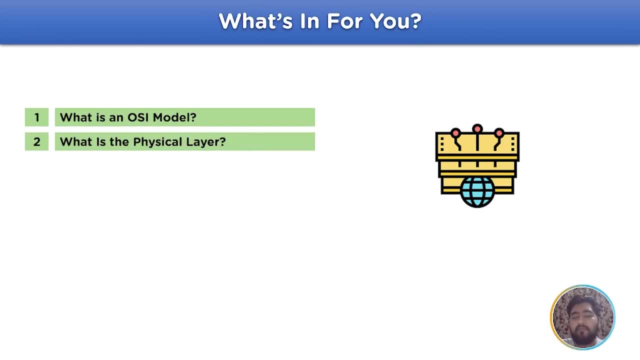 model of the OSR model, Advancing with the core topic, that is, what is the physical layer in the OSR model, Moving on with the attributes of the physical layer. Finally, we will wrap up our session by discussing the critical roles and the importance of physical layer. 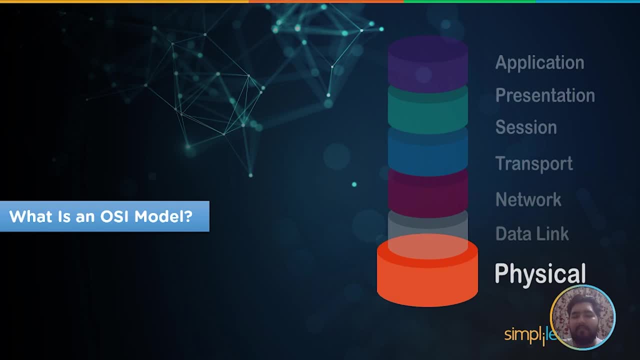 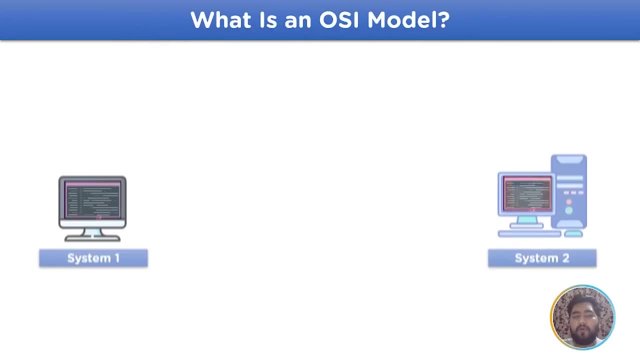 in the OSR model. Now let's get started with the first topic, that is, what is an OSR model? To better understand the OSR model's role in transmitting data from a network to another, let's consider we have two networking devices between which data is being transferred. The path between: 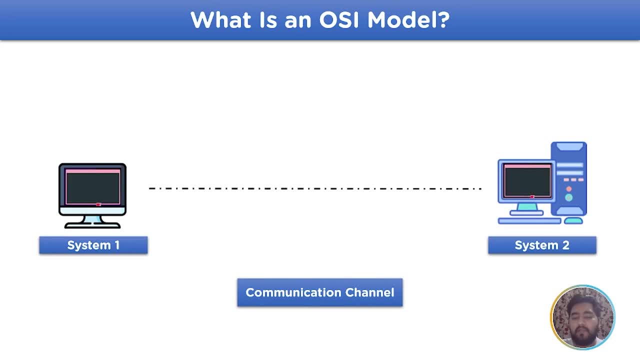 the devices is called communication channel. Let us assume that we different operating system for the network channel. To overcome such situation, we need to understand the role of the OSR model. To understand the role of the OSR model, we need to understand the role of the OSR model. Let's consider: 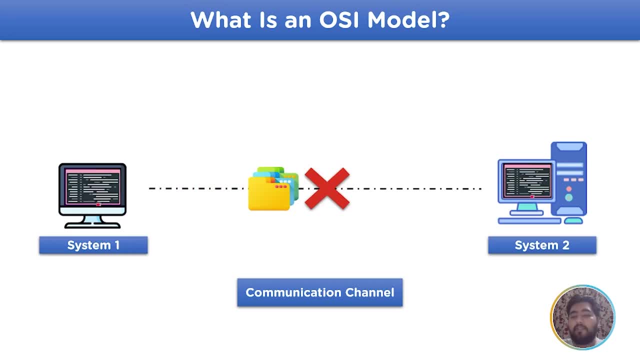 where the data cannot be transferred due to the different OS in the system, OSI model is used, which uses the seven layer structure to allow that conversion of data from the upper model to the data that is to be transferred. Now let's take a look at the technical definition of the OSI model. The OSI model stands for: 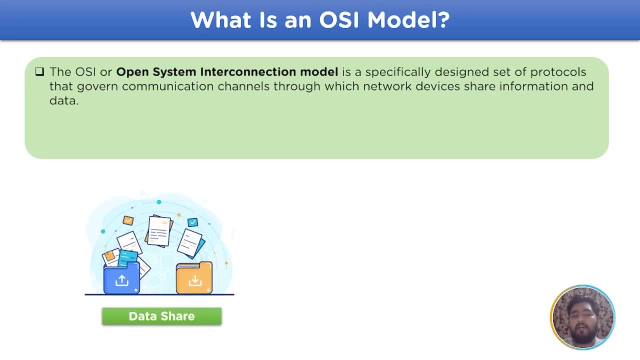 open system interconnection model A specifically designed set of protocols and standards governing the data's modeling and conversion of proper transmission. The OSI model is divided into seven layers which perform specific functions and apply protocols to maintain data quality without any error. Now let's move on to the main heading for the session, that is what is a. 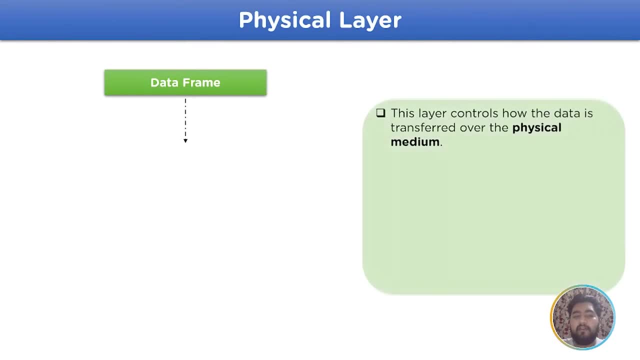 physical layer. The physical layer which provides and is responsible for physical mode between the sender and the receiver node in the data transmission. This layer converts frames received from the data link layer into bits, that is, in terms of ones and zeros to be transferred. It is also responsible for 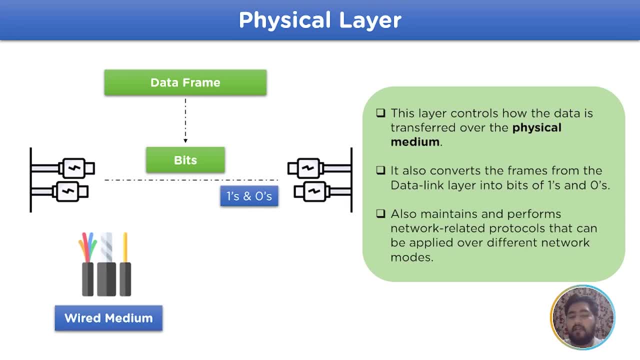 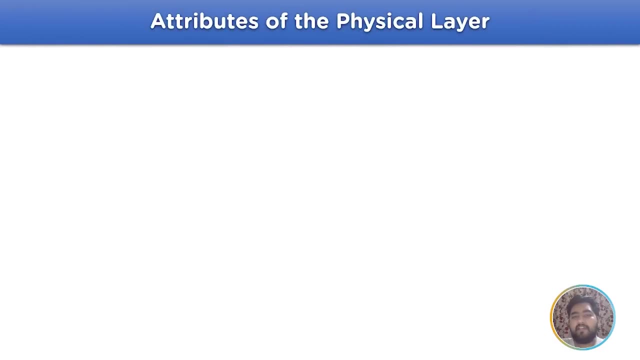 maintaining the data quality by applying necessary protocols and maintaining the bit rate through the data transfer using wired and wireless medium. Now let's move on to the attributes of the physical layer. The physical layer has a multiple attributes, which is applies in the OSI model. The first is signals. The 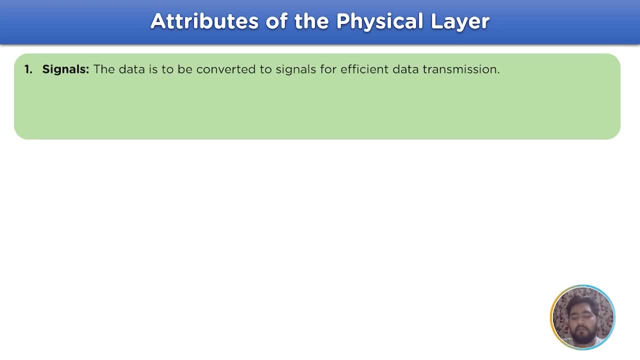 data is to be converted to signals for efficient data transmission where it has two different types. Digital signals represents the network pulses and digital data from the upper layer, whereas the analog signal is converted data for transmission of the model. The next attribute is known as transmission. 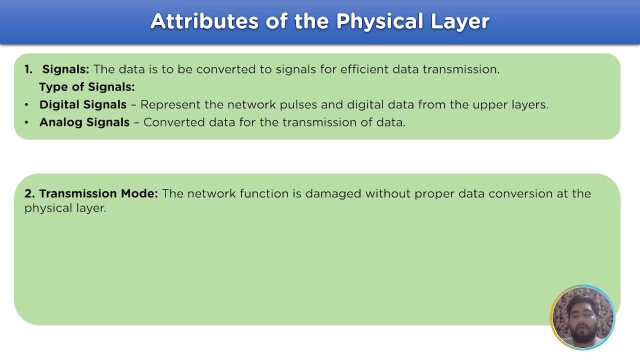 medium. The network function is damaged without proper conversion at the physical layer. It has two different types: Wired medium: The connection established is made through application of cables- Example: fiber optic cable and coaxial cable. and the second type is wireless medium, Connection established using the wireless communication network- Example: 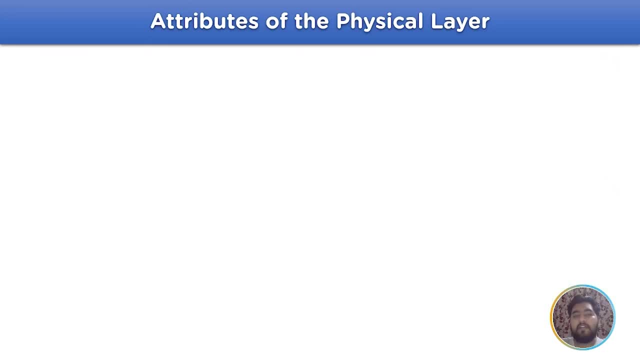 Bluetooth and Wi-Fi. The other attributes of the physical layer are data flow, which is defined as the rate of information flow, and the transmission wireframe. The factors that affect data flow rate are error rate, Receiving incorrect data due to noise in the transmission. Encoding: Encoding data. 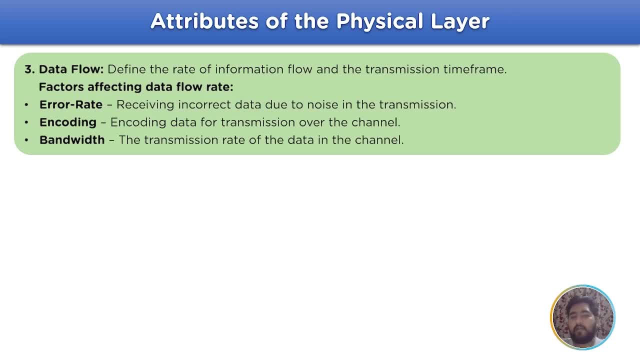 for transmission over the network channel. and the last is bandwidth, That is, the transmission rate of data in the channel. The last attribute of the physical layer is noise in transmission. During data transmission, the transmitted data may get damaged or corrupted due to multiple reasons, Some of which are mentioned as dispersion In this case.